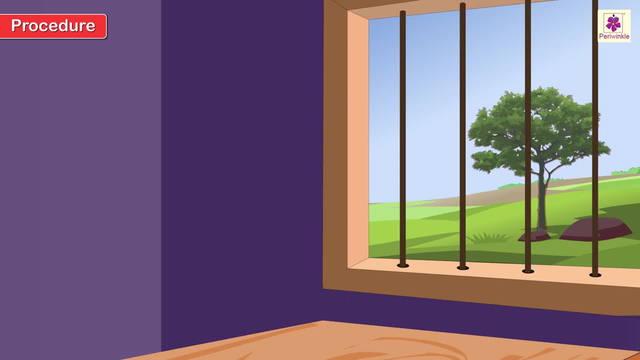 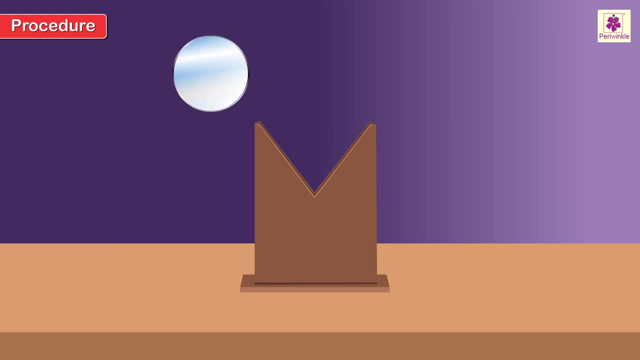 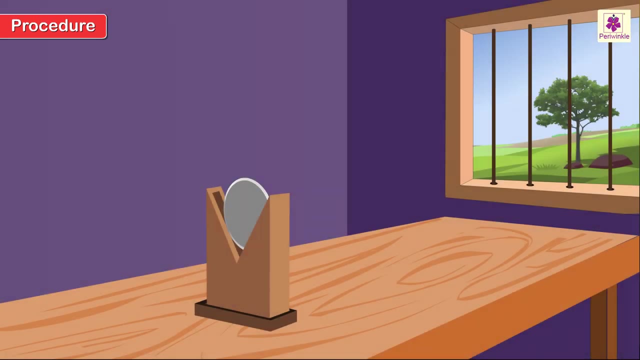 For example, we shall consider this tree. Step 2: Place a concave mirror on its stand and put it on a table so that its reflecting surface is facing down 22.. Step 3: Place a screen fixed to a stand on the table so that the planes of the screen and mirror 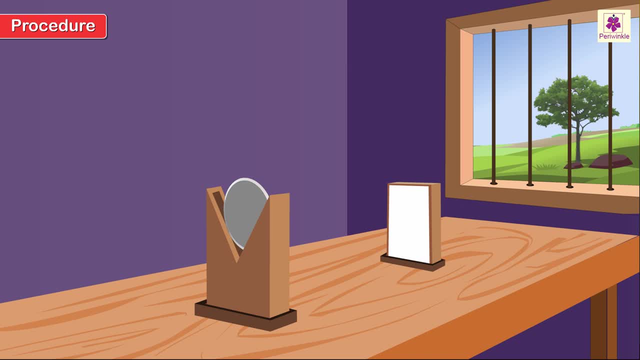 lie parallel to each other, Mr Moving of the screen to and fro, so that the distance between the considering a concave mirror- 500 degrees here- is least than the distance between it and the���ерж mirror is either decreases or increases. this shall not happen. 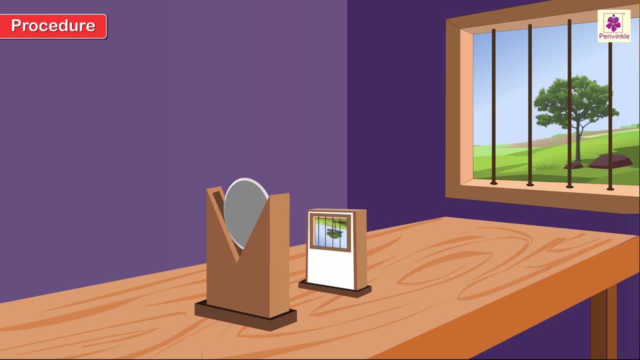 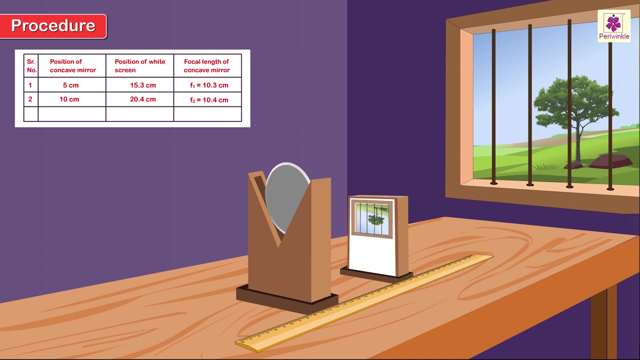 till you obtain a sharp inverted image of the object on the screen. Step 5: Using a meter scale, accurately measure the distance between the pole of the mirror and the screen. Step 6: Record the distance as F1.. Step 7: Repeat the earlier steps twice to obtain two more readings, F2 and F3.. 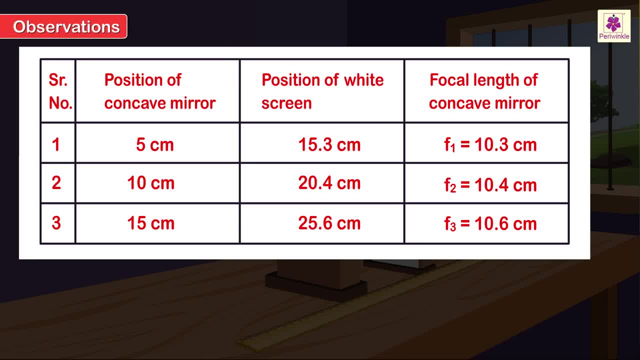 Observations: When the position of concave mirror is 5 cm and the position of the white screen is 15.3 cm, the focal length of the concave mirror is 10.3 cm. When the position of concave mirror is 10 cm and the position of the white screen is 20.4 cm, 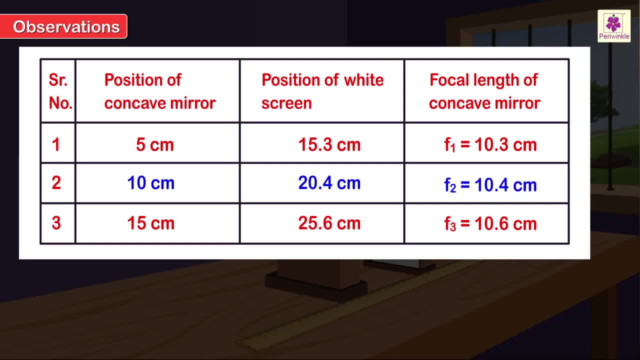 the focal length of the concave mirror is 10.4 cm. When the position of concave mirror is 10.4 cm, the focal length of the concave mirror is 15 cm and the position of the white screen is 25.6 cm. 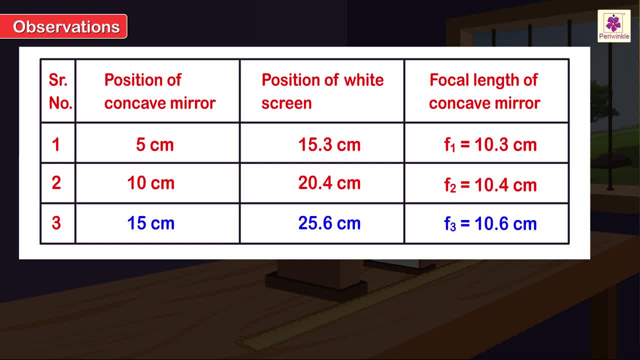 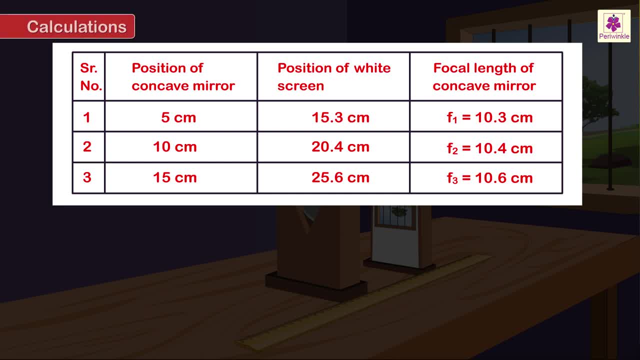 the focal length of the concave mirror is 10.6 cm. Find the mean focal length of the mirror. Calculations: Mean focal length is equal to F1 plus F2 plus F3. the whole upon 3 is equal to 10.3.